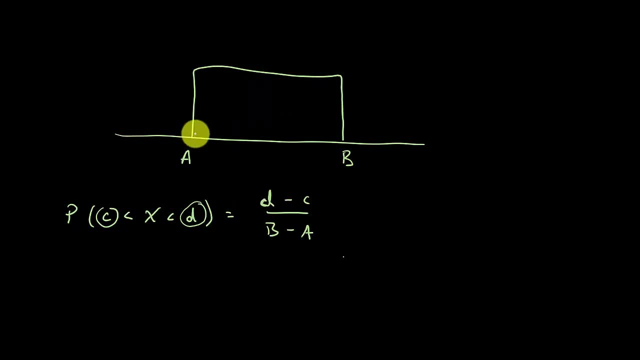 this curve. okay, and remember, for a uniform, well, for any probability distribution function, the area under this entire curve. here, okay, no matter what a to b are the area under the entire curve, that's one, all right, so let's go ahead and get started. so it says: suppose x is a random variable, that 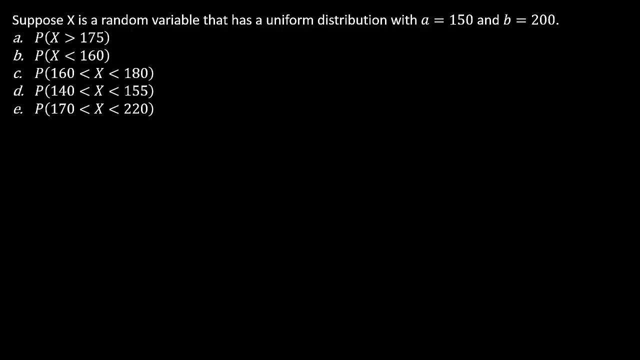 has a uniform distribution with a equals 150 and b equals 200. all right, so i know, over at the first they had, you know, it showed it with capital a, capital b, and here it's lowercase a, lowercase b. that's fine, okay, that's fine, but this is the minimum value that it can take on, and this is 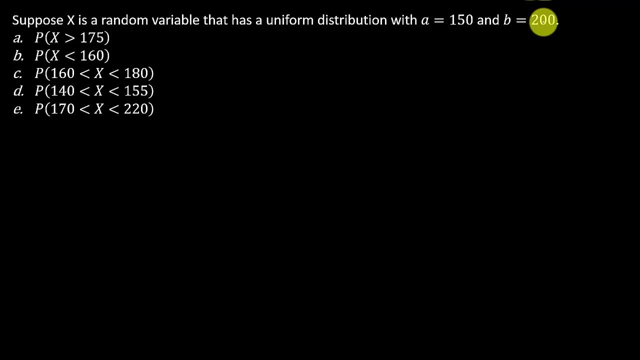 the maximum value, all right. so first let's look at part a. all right now. what i would recommend whenever you're doing these problems is: draw the picture, okay, draw it out, all right. so there's my minimum and maximum value, so let's just go ahead and draw. 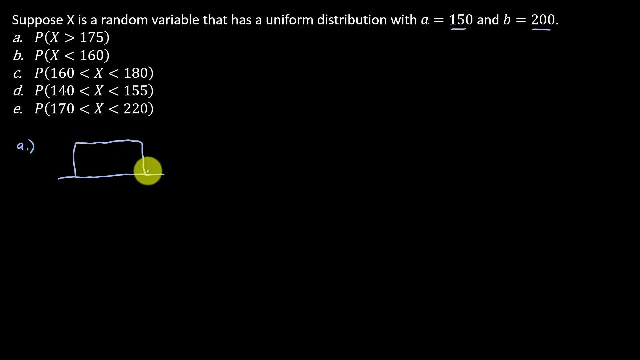 this out, all right. so here we've got 150 and there we've got 200, all right, so we're looking for the probability that x is greater than 175, all right, so what i would do is i would put 175 in here and draw in what we're looking for? well, we're looking for the 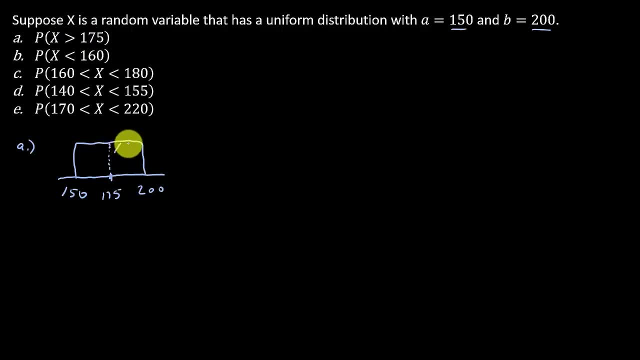 probability that x is greater than 175. so that's this area here all right now, i know, with the probability of 175 you're looking well in that area from here all the way, all the way out here to infinity. yeah, that's what they're looking for, but in this uniform distribution. 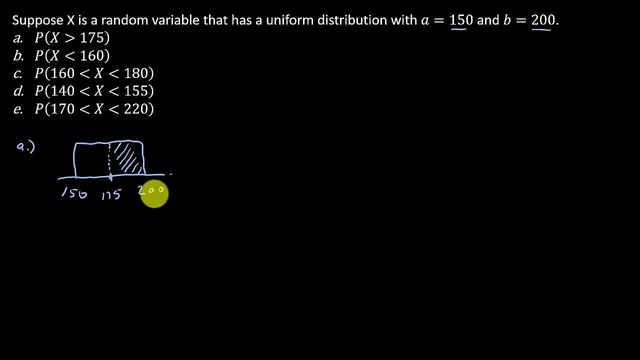 the maximum value that x can take on is 200. all right, so once we get outside here, okay, all this stuff over here. let me get a different color and show you. so all this stuff out here. well, remember, the probability is the area under this curve. well, all this probability out here. 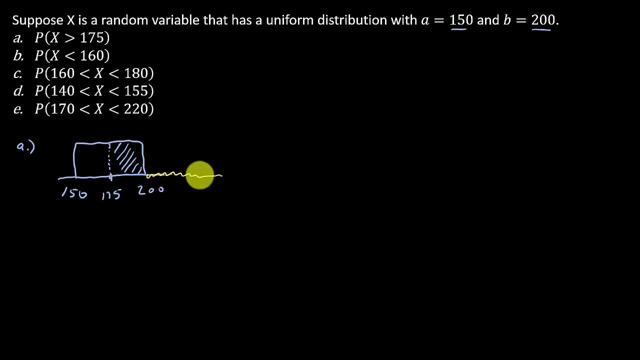 well, there's no height here, right? that area there is zero. okay, so the probability that x is greater than 175 would be 175 to infinity. so it would be this area plus the area from here to infinity which would be zero. so it's just this area, all right. so i'm not going to go. 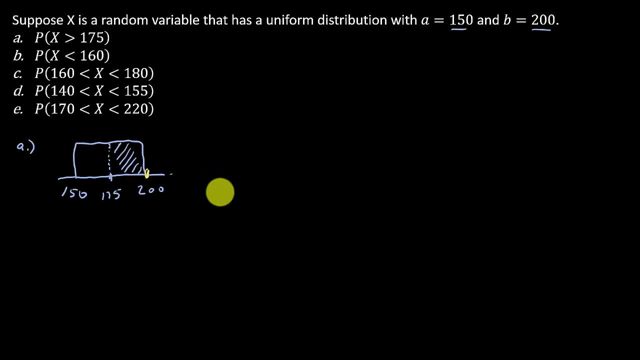 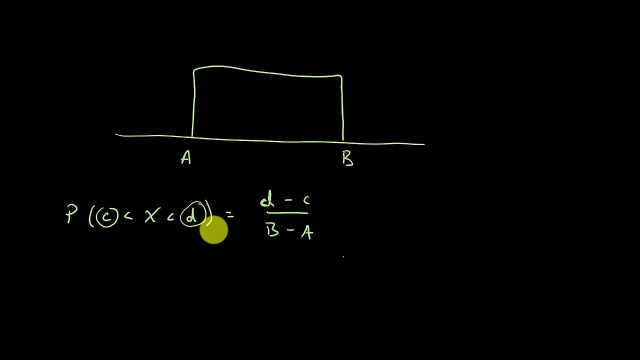 over that every time, but i just wanted you to make sure, on this one, that you you know you understand what's going on. all right, so let's go ahead and find this probability, so the probability that x greater than 175. all right, so remember it's. it was this between the two numbers. all right, 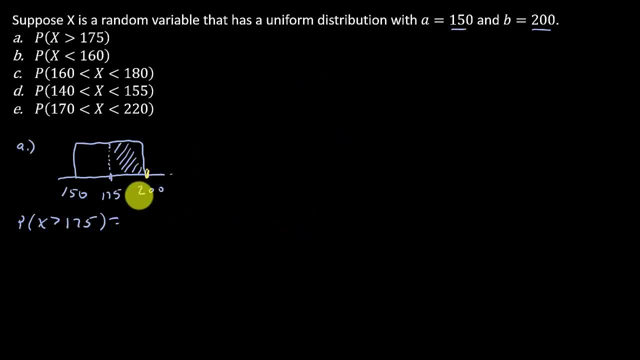 all right, so this is going to be 200, see, because that's the maximum value, just like. look, just like in the in the problem i had earlier a, b and remember the probability c less than x less than d. remember that probability was d minus c over b minus a. okay, so that's the maximum. 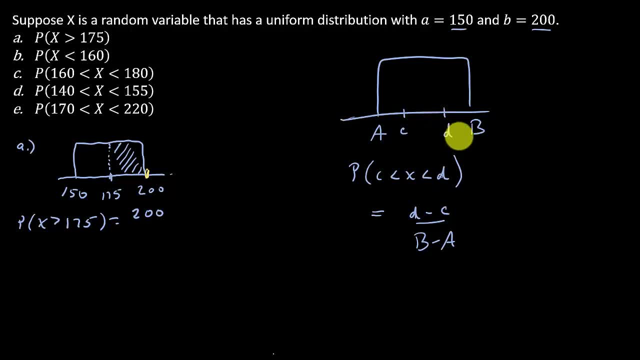 value. so see, it would be two numbers in here: the maximum value minus the minimum that gives us the numerator, and then the maximum value and the minimum value that the distribution can take on. okay, so b minus a, all right, so in this case, yeah, it's greater than 175, but we've got to stop here at 200. okay, so in this case, 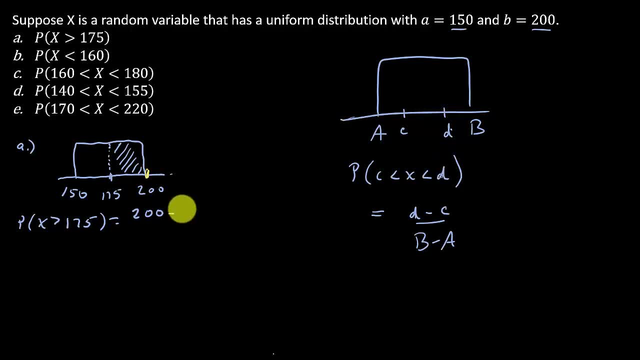 d is 200, so that's 200 minus 175 over 200 minus 150, and so that is going to give us what? 25 over 50, which is one half, all right, all right. so let's take a look at the, at the next one. 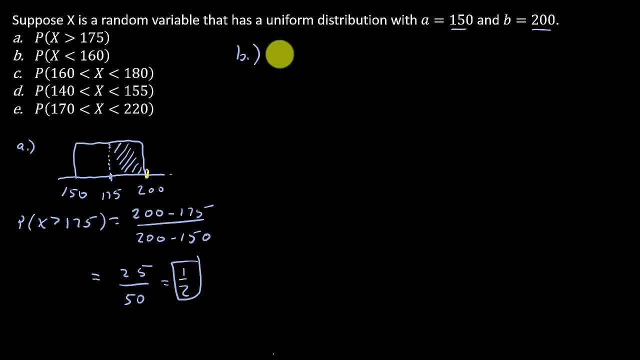 let's look at part b. so we've got the probability that x is less than 160.. all right, so let's draw the picture and draw in the 160 here and we're looking for what? that it's less than 160.. so that means everything to this side, all right. so i'm not going to spend time about explaining all. 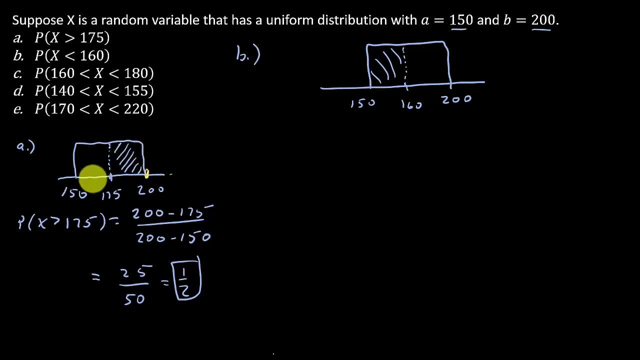 the probability out here. that's why i did it here. okay, so this is the same reasoning. it keeps going, but we have to stop at the 150.. so the probability that x is less. i'm sorry, yeah, i started stop at the 150.. x is less than 160.. well, that's what the larger 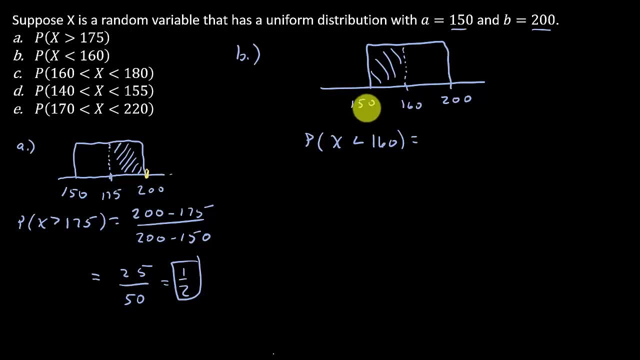 well, that's what the larger. well, that's what, the larger minus the smaller. this is what we're finding: the probability between 150 and 160.. so that's 160 minus 150 over 200 minus 150, and so remember the big capital a and b here. so that's going to be. 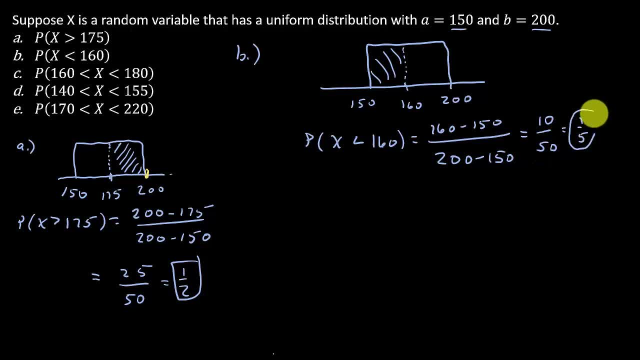 10 over 50, which is one-fifth. all right, let's take a look at the next one. all right, so the the next one is which z hundred and maneuverable, half of z here, and then weそう here and we can completed 100, you know, and you put in the table, and then we have a 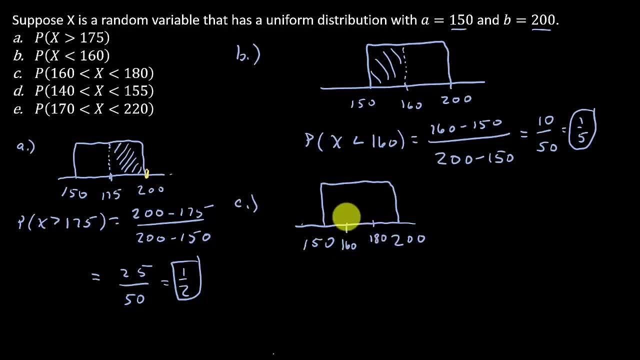 z and a half. here we'll just make a conclusion that z and a half is equal to the power of a five in the next window, and we can say that z is less than 160.. would be that area there, so the probability would be what? well, the 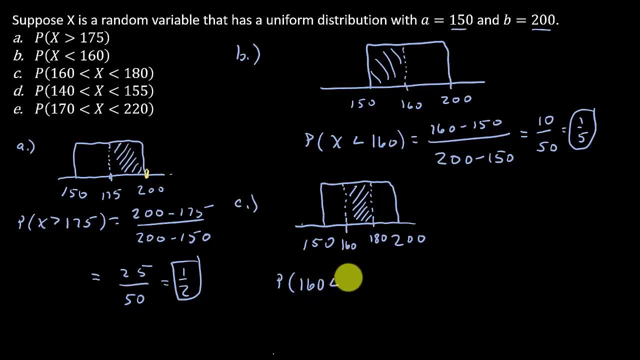 probability that let's see 160 less than X, less than 180. so that's going to be what: 180 minus 160 over 200 minus 150, and so that's going to be what: 20 over 50, which is two-fifths, all right. so we got two more and I'm all race this. I'll 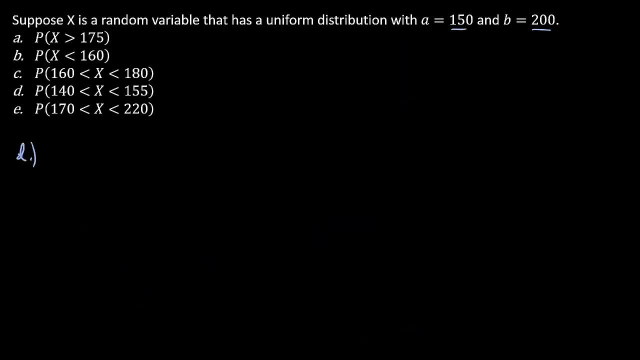 pause it while I erase it. all right, so let's look at Part D. all right, so we got probability that X is between 140 and 155. all right, so let's draw this, so you let's see I've got what. 150 and 200, that's my max and min values and I want 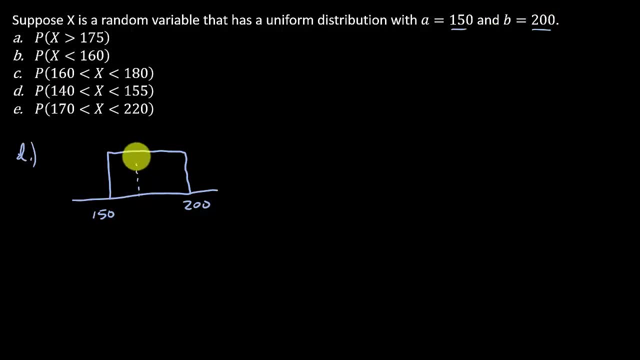 to find the probability, let's see 155 and 140. oh well, 140 is out here, but we can only go to 150. all right, so the probability that X is between 150 and 150 is a probability that X is between 140 and 150. this means: 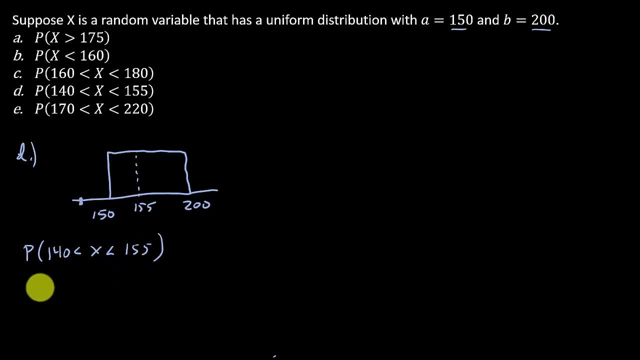 that X is their maximum and they are going to be between 150 and 150. so we that X is their maximum and they are going to be between 150 and 150, and 150, 140 and 155. all right, we're looking for this area, so it's gonna be this area. 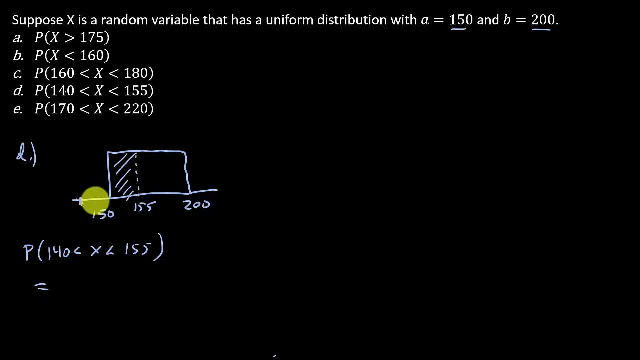 plus the area from here to here which we talked about earlier. that area there is zero, so we don't have to mess with it. so we're just gonna find the probability between 150 and 155. so that's gonna be 155 minus 150 over 200 minus 150, and